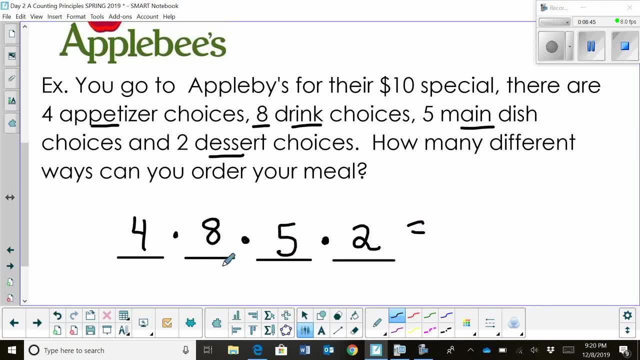 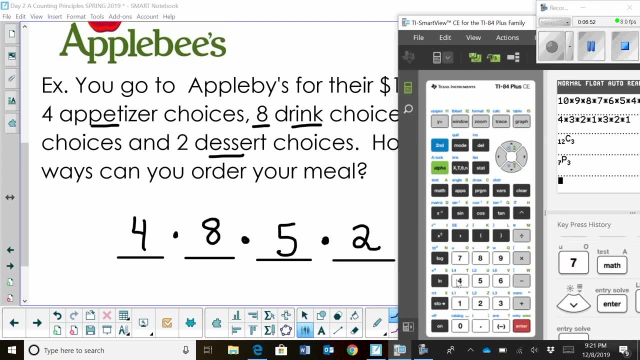 desserts. Now for the counting principle. all I do is multiply all these together. So let's grab my handy dandy calculator and I'm going to multiply it together Four times eight times, five times two. Then I get- Let me pull this back out- 320 different ways I can go to Applebee's for my. 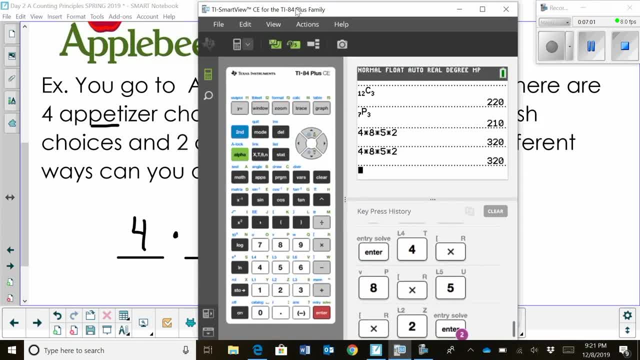 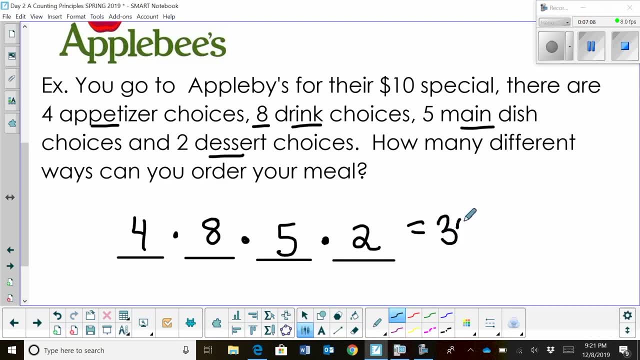 herbal juice, the one I have right now, because I like to drink this with ice cream. But after all this Brouryu you had earlier on the food, I just need to charging it. So are you buying a glass of be Applebee's and get a meal? three hundred and twenty eight twenty different ways, so I could. 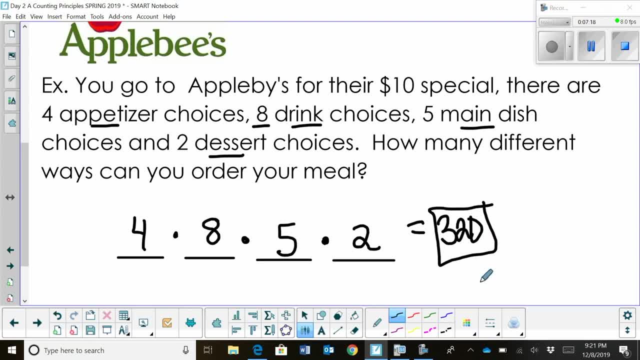 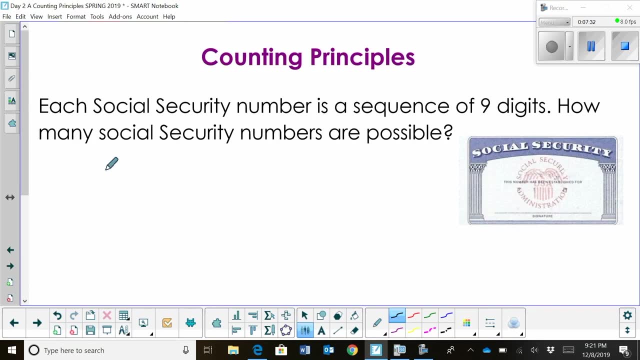 go almost every day the whole year and get an order from the menu and get a different common. they are different different meal every each of those times, so it's kind of interesting to see how many different ways you can do it. so let's look at a couple other counting principles. okay, 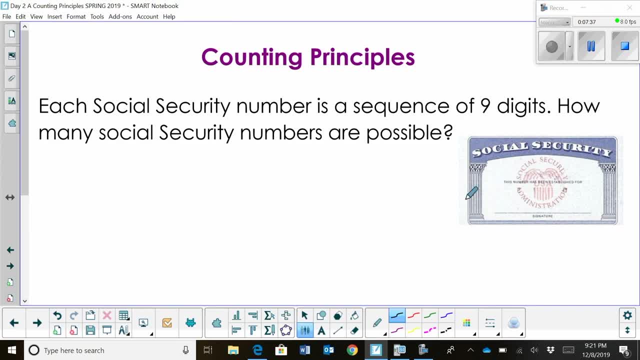 we've got a social security number. I think most of you have a social security number- and there are nine digits in that number. how many social security numbers are possible? well, you have to think. well, how many events do I have going on? I have nine events, one for each digit, so one, two. 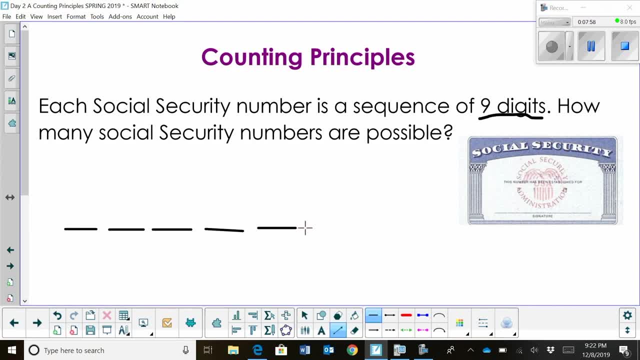 three, four, five, six, seven, eight, nine. I'm trying to draw straight. didn't draw straight, but that's all right. okay, then you are going to multiply all these events together. so I'm going to multiply these and I've got to start thinking: how many different possibilities, how many different ways can I pick the first digit? 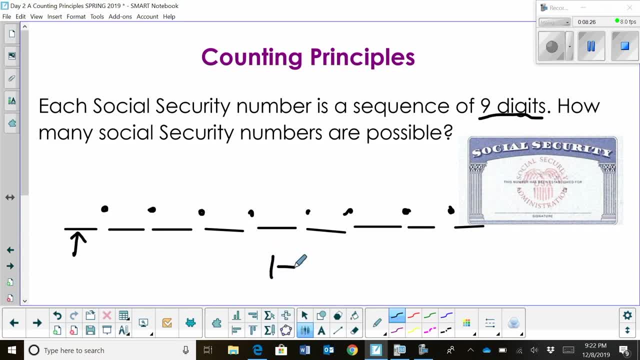 well, I have the numbers one through nine, plus we can't forget about the a zero. a zero counts also, so you actually have 10 different numbers to choose from, including zero. so the first digit could be zero. it doesn't say it can't be. so I have 10 choices. well, how many choices do I have for my? 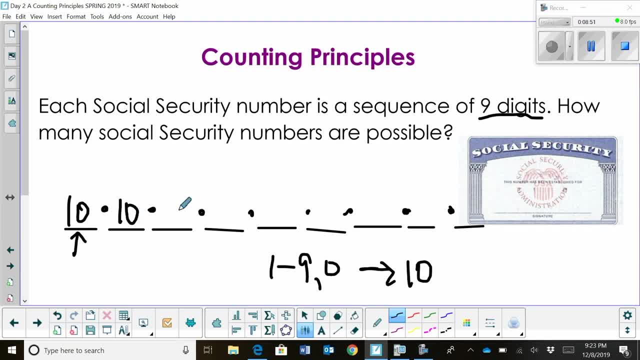 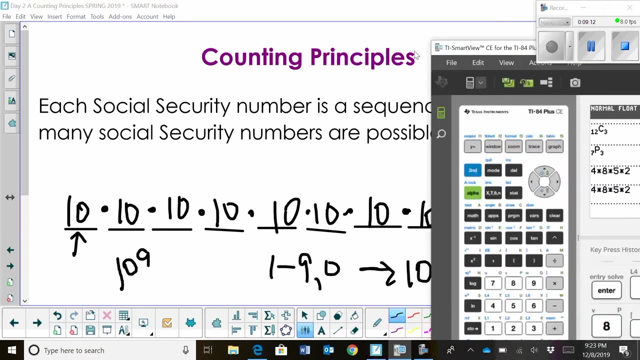 second digit, I have 10 more choices because I can repeat numbers, so I'm going to have 10 choices for all nine positions. so it's just going to be 10 times 10 times 10, nine times. okay, we can also write this as 10 whoops to the 9th, power 10 to the 9th. so let's grab our calculator and pull that. 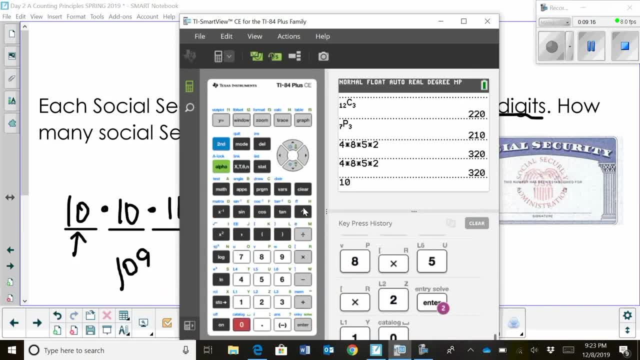 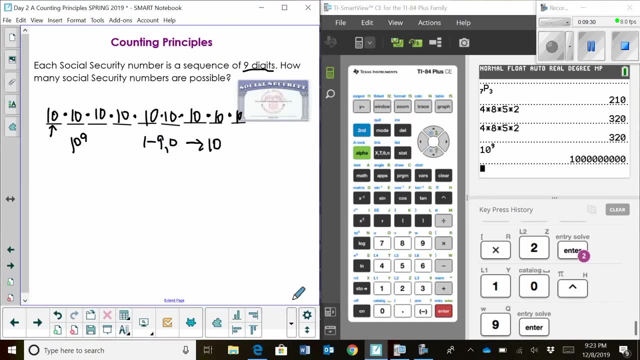 back out and we'll actually figure out how many social security numbers can be created. it's going to be a lot, wow. so I've got one with one, two, three, four, nine zeros after it. okay, so let's write that down. I should have known that. sorry about that, um. 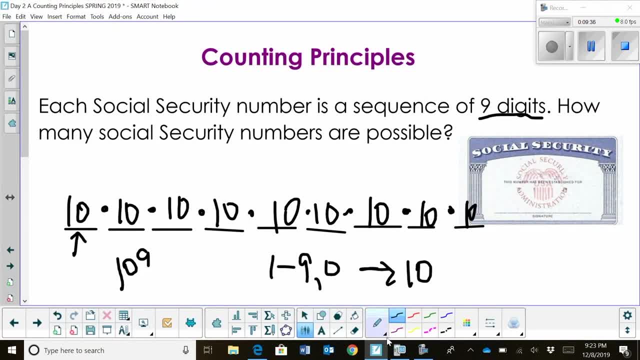 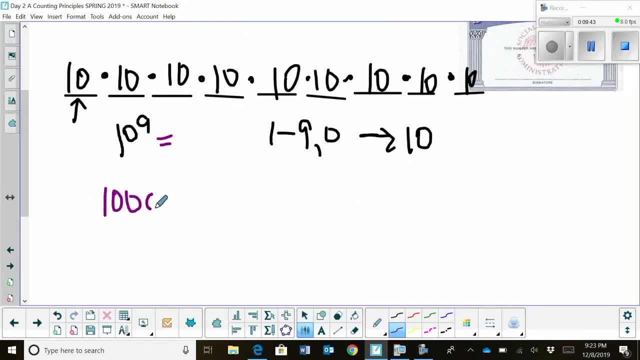 let me grab my pen here. whoops, grab my pen and I've got one, one, two, three, four, five, six, seven, eight, nine. so what's that? a billion different numbers. we have one billion different ways to give a social security number. so that's a lot. okay, let's try. 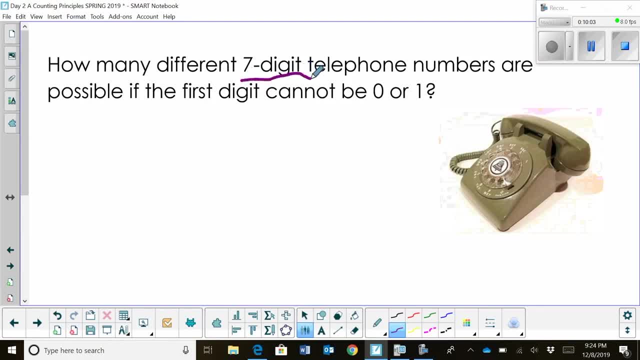 the phone number problem. okay, we have a seven digit phone number. how many are possible if the first digit cannot be a zero or one? we know if it's a zero that's going to call the operator, and if it's a one it's going to call long distance. so 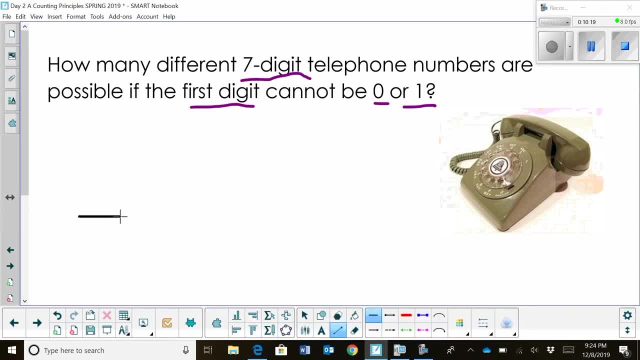 we have to eliminate those choices. so how many events do we have going on? well, we have three in the front, then we usually have a dash here and then four in the back. so we have seven different positions or seven events. how many possible outcomes? or how many ways can I pick the first digit if I can't use a zero or a one? 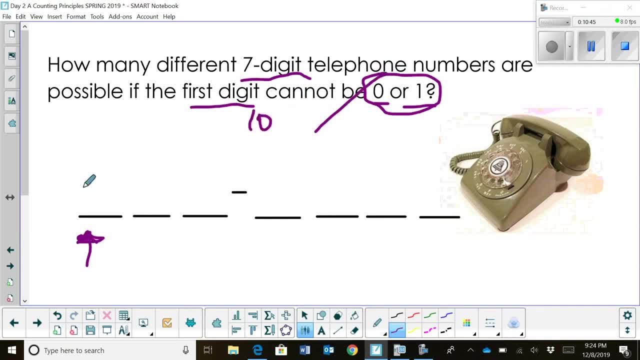 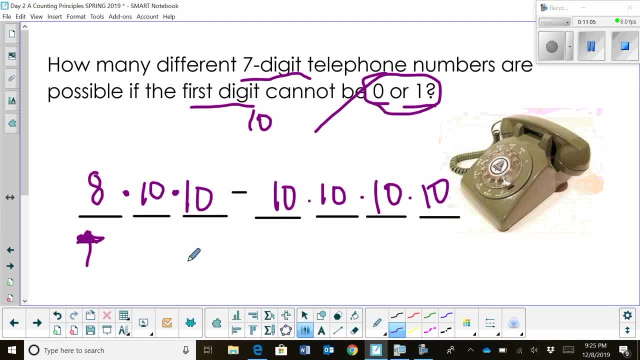 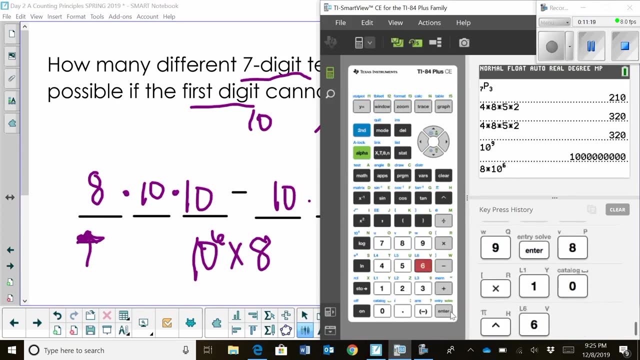 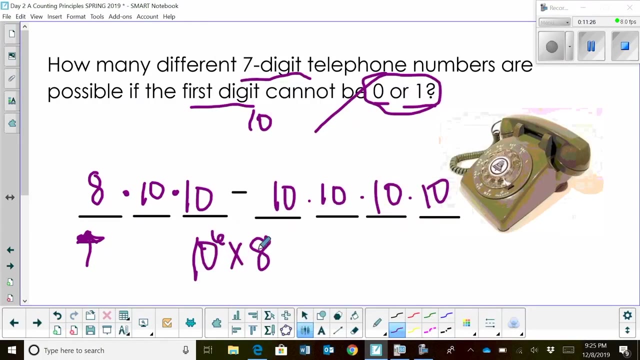 choices. so I have ten. what to the sixth power? all times eight. so what's ten to the six times eight? let's take eight times ten to the sixth power and boom, I have what's that? one, two, three, eight million different ways. yep, eight million, that makes sense. I would have eight million different phone numbers. 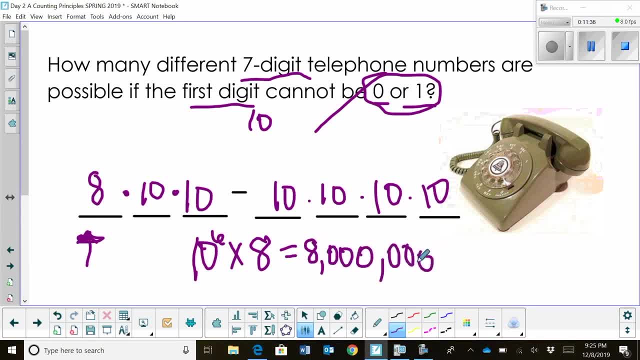 now, as you know, there are probably more than eight million phone numbers in the world, so we have to add area codes that are three digits, and that adds a whole bunch more possibilities. so you could figure that out too, if you wanted to. okay, let's see how this problem's slightly different. 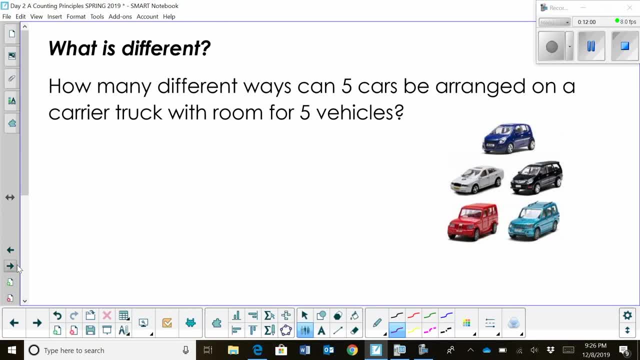 but we can still use the counting principle. okay, how many different ways can five cars be arranged on a car carrier truck with room for five vehicles? so let's just think about what we have. we have one of these trucks that has a top floor and a bottom floor, and then it's got an 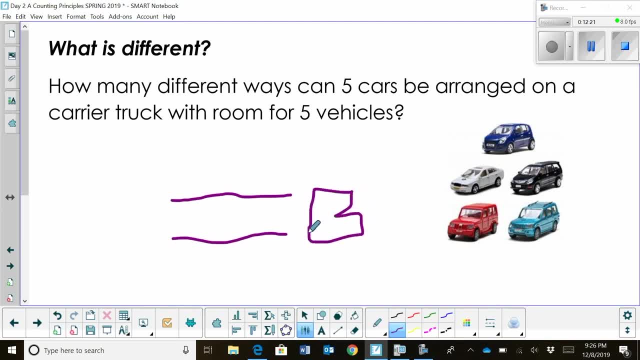 engine up here. I like to draw a little picture of it. okay, and here's the front light and here's where the driver is. okay, and he it needs to load cars up here. well, we have a spot for one, two, three, four, five cars, something like that. there may be three on top and two on the 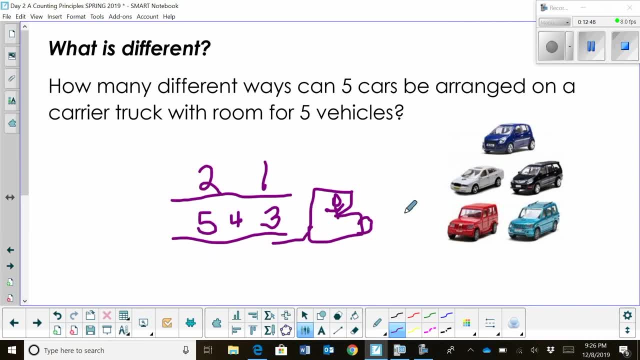 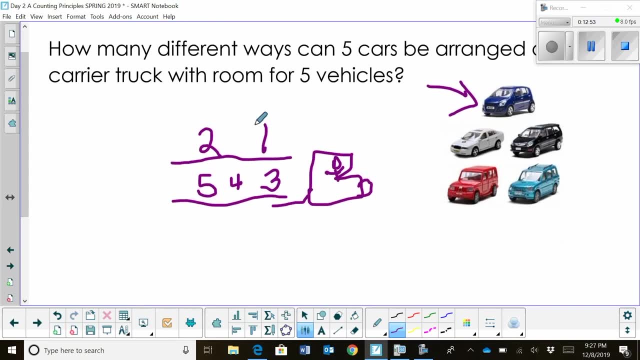 bottom, but anyway, we have a spot for five cars. how many different ways could we arrange these five cars? well, what's different about this is, once we place a car, we can't use it again because we've already placed it. so we have to think about our five events. we have five events going on because 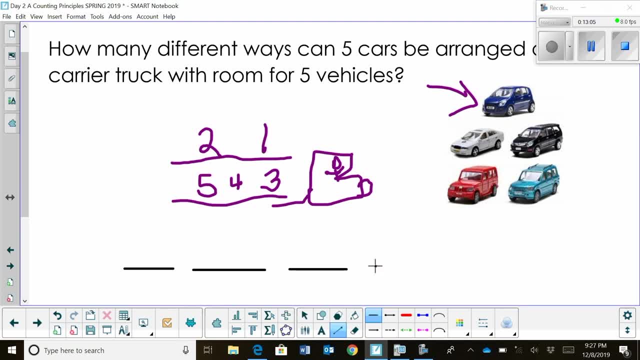 we have five positions for five cars, so let's draw our five lines to represent each event. okay, now for spot one. how many different cars can we put up if we have these five cars lined up? well, we could pick any of them, so we would have five choices. but then, for the second position, once we've put a car, let's just